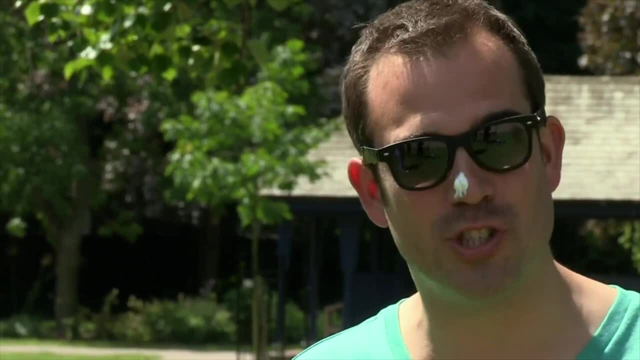 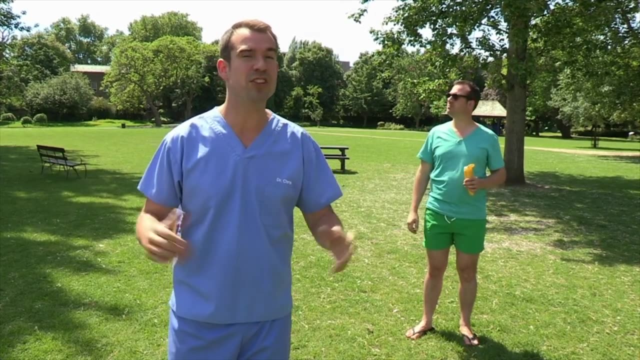 hot, hot, hot, And I always like to be the first to break out the shorts and sun cream. Erm, you've missed a bit, But you never know how long the sunshine is going to last. At any moment the sun could go in. I don't think so, Chris. it's actually quite a nice day. 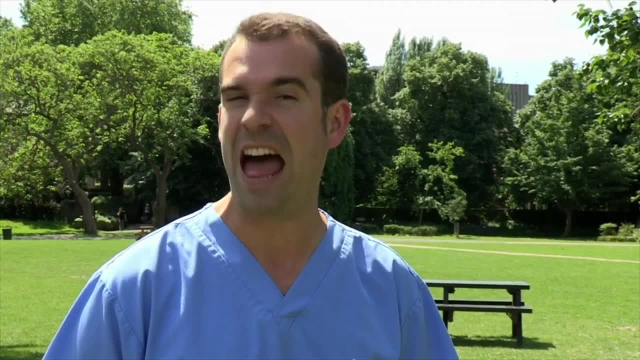 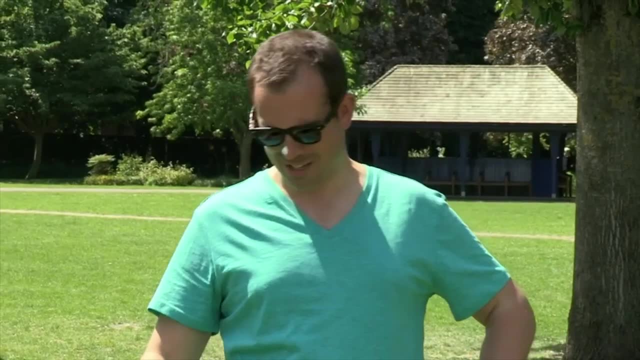 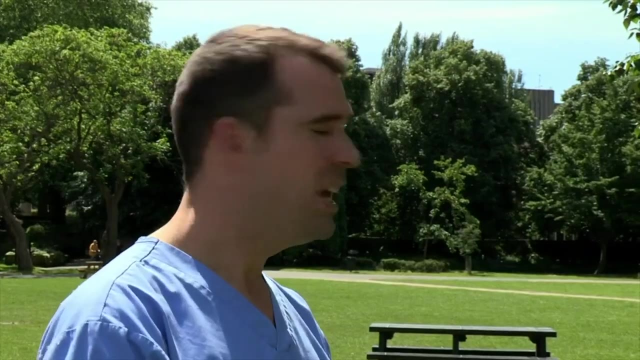 And once the sun's gone in, it could start getting chilly and that could be dangerous. At any moment it could bucket down with rain. Well, actually, Chris, I did bring an umbrella for that very eventuality, And in this country, even on a day like 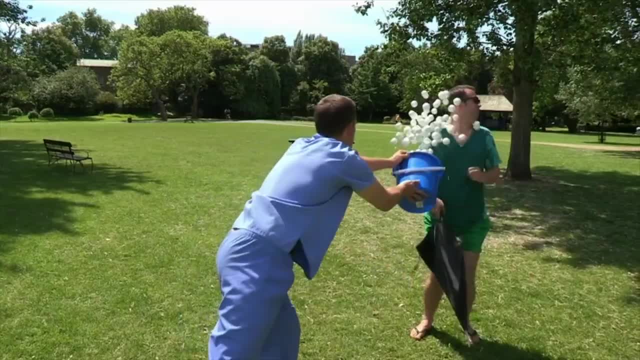 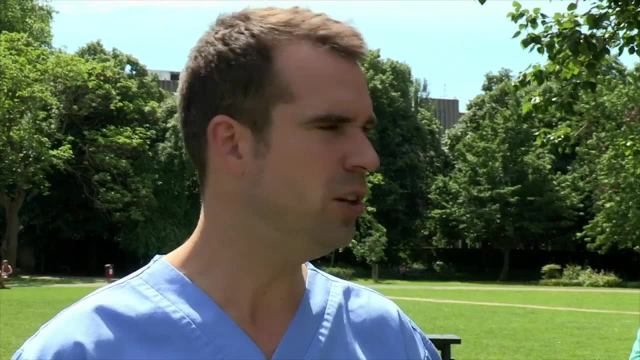 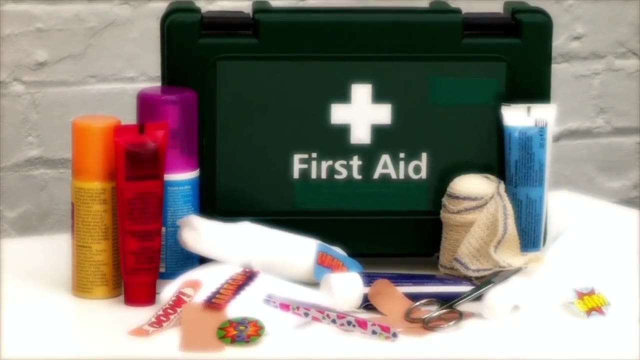 today it could hail Hail, Which is why you should always pack an extra layer of dry clothes, isn't it? Zand, Zand, Uh-oh, Zand's gone, pale and unresponsive. This looks like hypothermia. 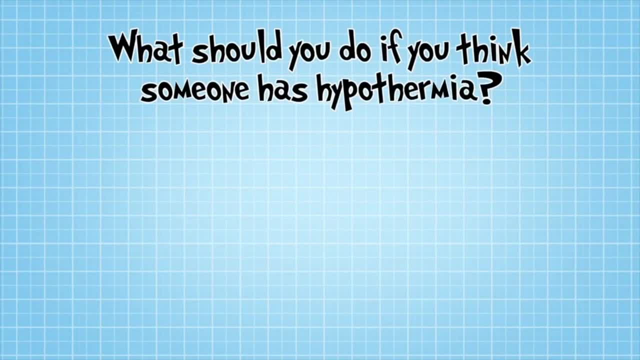 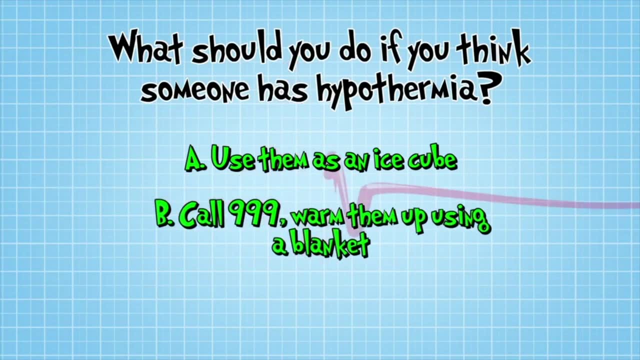 So what should you do if someone is really cold and you think they may have hypothermia? A- Use them as a giant ice cube in your drink. B- Call 999.. 999, warm the person by wrapping them in a blanket and give them warm drinks and chocolate. 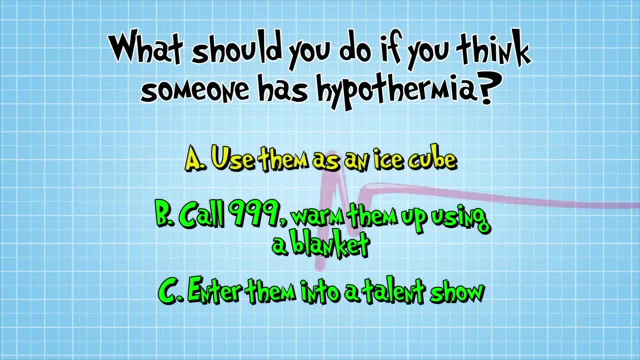 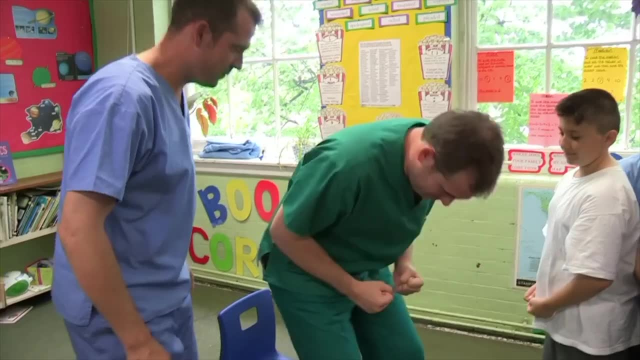 Or C- Enter them into a talent show as a novelty shivering act. What do this lot think? B- Wrap them in a blanket and call 999.. Emily's absolutely right. Have a look at this. Let's take you down Now. how cold are you? I'm freezing. 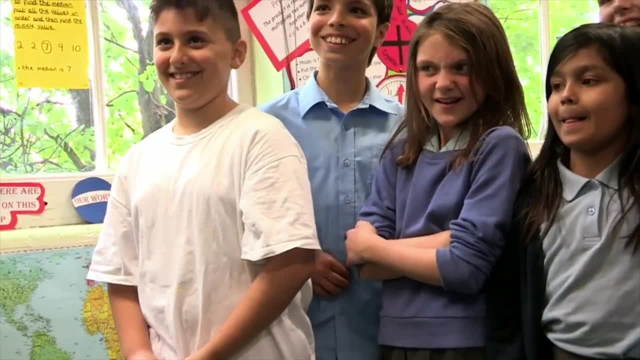 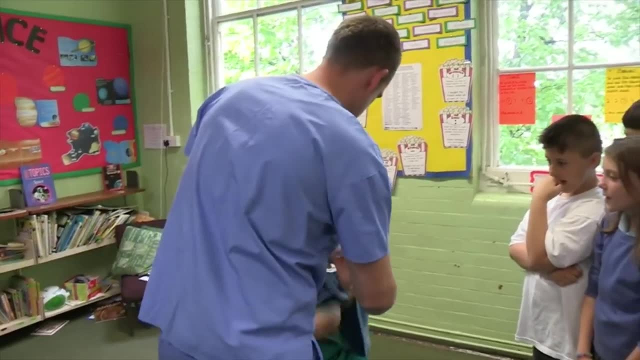 Are your lips blue? Yeah, blue lips. Do you think your lips are blue? Yes, Yes, his lips are blue. Yes, his lips are blue. Yes, his lips are blue. Let's get you a blanket. Also, we can give him a hot drink and chocolate ball. 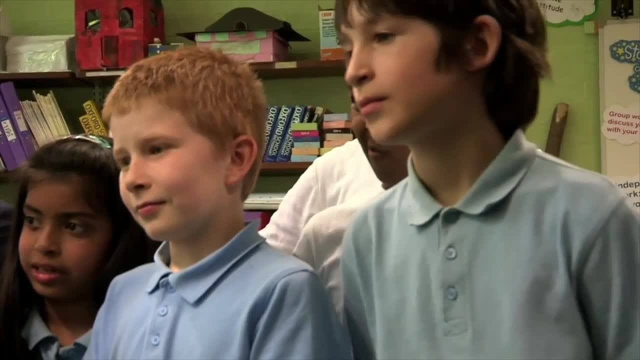 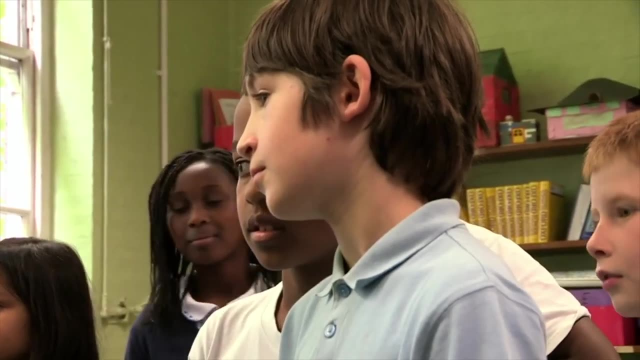 Sometimes the person may even be confused. So do you know who you are? I'm Dr Chris. Oh dear, looks like he's a bit confused and he's not going to be able to warm himself up, even with a blanket or with the tea. I think we need more help. 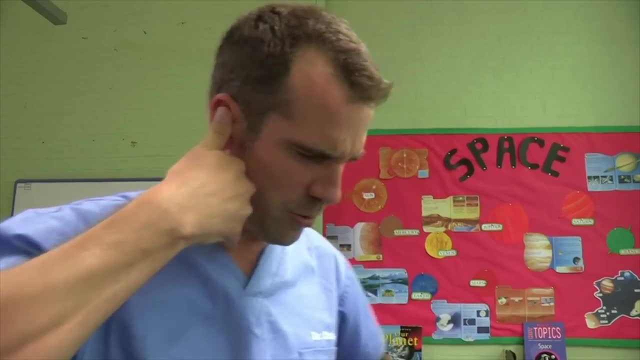 Ring, ring, Ring, ring. Emergency services. what's the problem? I thought you were hypothermic. I'm just doing the emergency services bit. Oh, I see, Okay. okay, It's Dr Chris here. I've got an emergency. 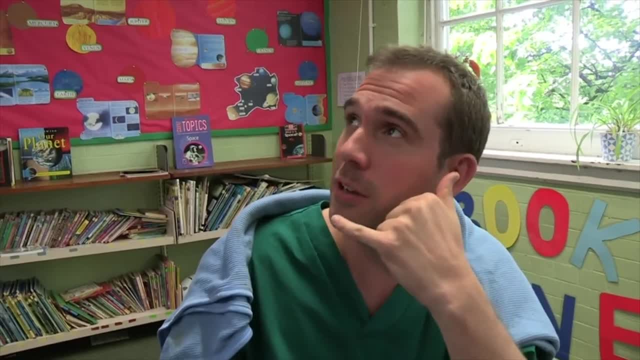 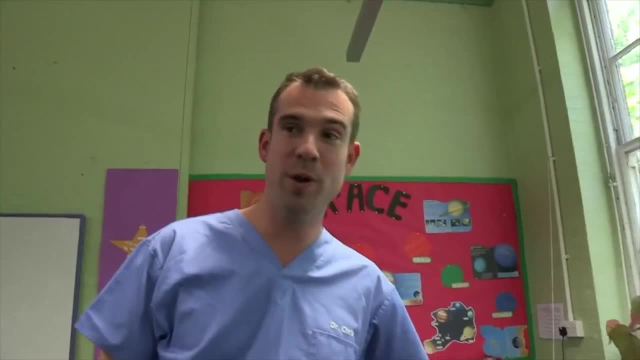 I want the ambulance please. Oh right, Whereabouts are you? I'm at the Operation Out School. We'll get an ambulance to you straight away, Thank you. So now we'll just look after you and, if we can, we'll take off his wet clothes and move.